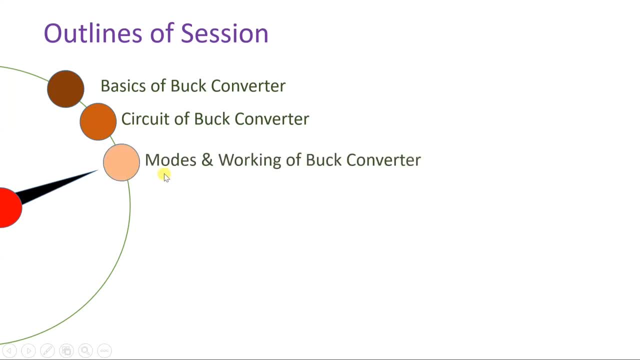 explain circuit of buck converter. Then after we will see different modes of buck converter and along with that we will see it's working. And then after I'll show you waveforms of buck converter and based on waveforms and working, we will see parameters of buck converter. 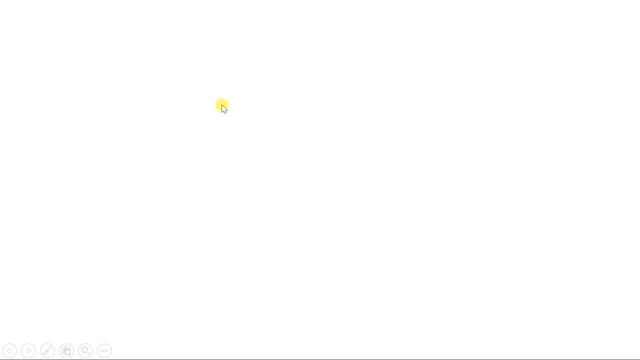 So let us begin this session with first agenda, that is, basics of buck converter. Now see buck converter, that is step down DC to DC converter. So here buck converter is step down DC to DC And, as its name suggests, buck means step down. Step down means voltage will decrease. 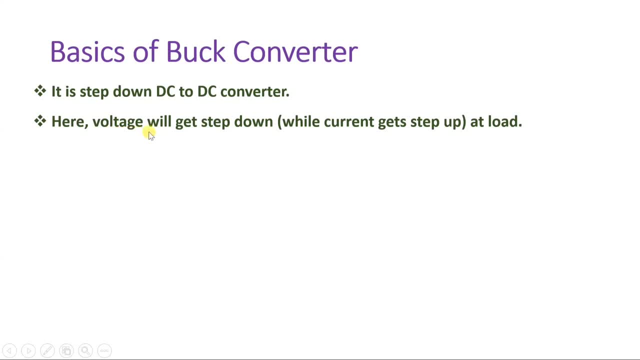 So here at output side you will be observing voltages less compared to input voltage at load side, And as we decrease voltage there will be increase in current. So current gets step up in buck converter. Buck converter can be very highly efficient and that efficiency could be greater than 90 percentage And because of that we 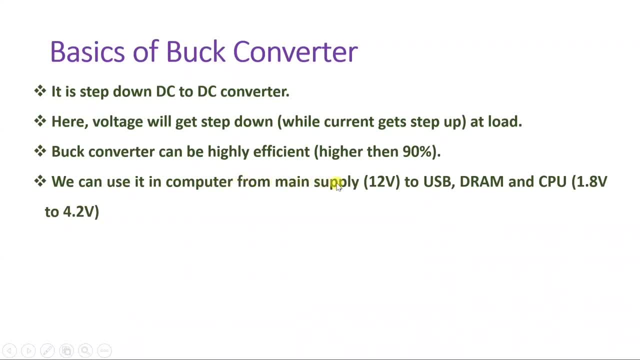 use buck converter in computer from main supply with 12 voltage to different elements like USB, dynamic RAM or CPU And that has been functioning at the voltage 1.8 to 4.2 voltage. So here main supply that is there with 12 voltage and that supply is being distributed. 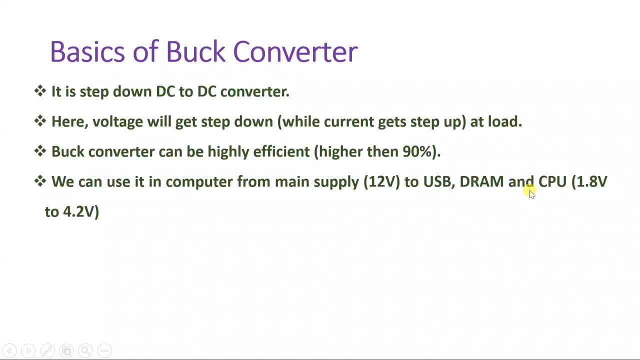 to different elements Like USB, dynamic RAM and CPU, which is functioning with the different voltage ranges from 1.8 voltage to 4.2 voltages. So that is where we use buck converter and by using buck converter even we can make effective SMPS. So switch mode power supply that even can be made by. 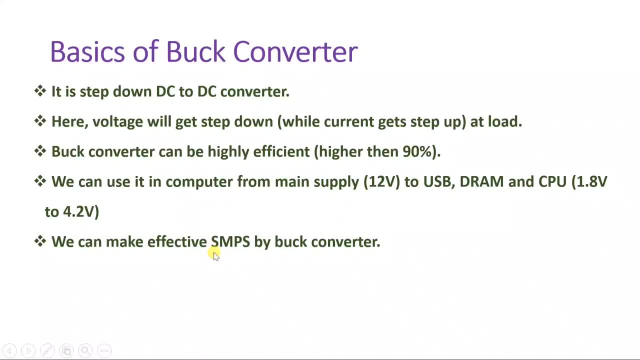 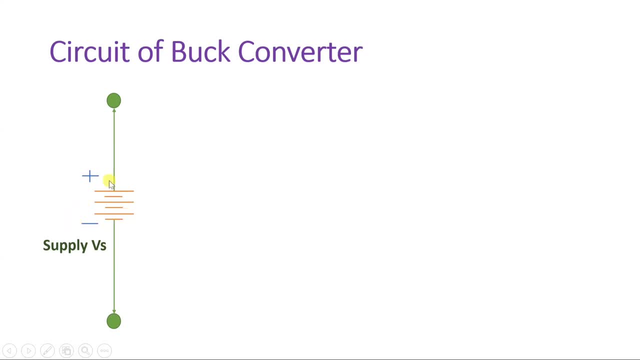 using buck converter. So these are the basics. Let us try to understand basic circuit which is there with buck converter. So as if you see Here we have a circuit, Then here we have DC supply. So this DC supply that we are delivered. 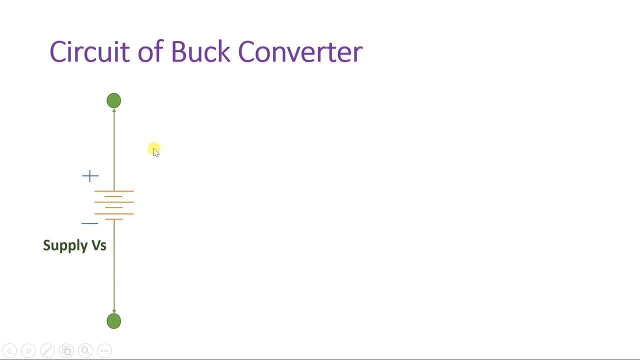 to utilize in buck converter where at load side, by using this circuit, we will be having less voltage. So here we use one switch, Here we have freewheeling diode, Here we are connecting inductor in series with load, where across load we connect one capacitor and here we 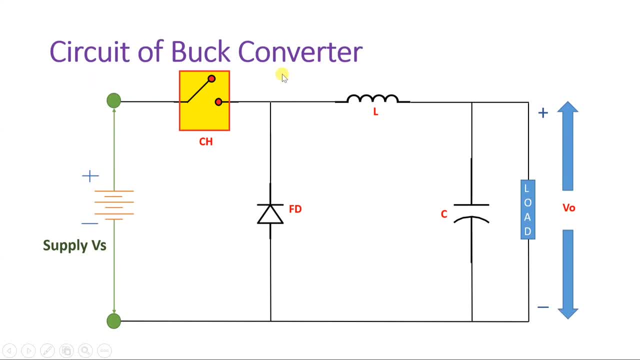 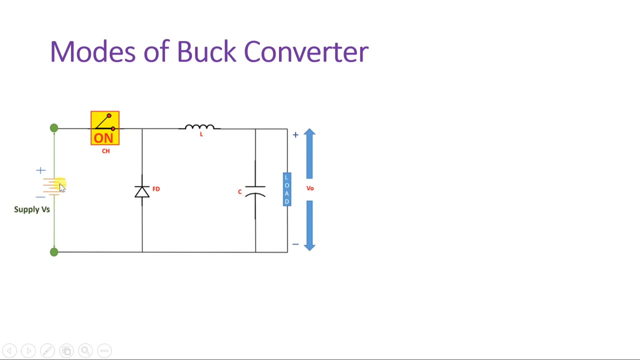 are taking our output voltage. So in buck converter you will be observing there will be less average output DC voltage compared to supply voltage Vs. So let us try to understand how this buck converter functions. So, as I have told you, this is the basic circuit in which there are two modes. In one mode, switch will be on and 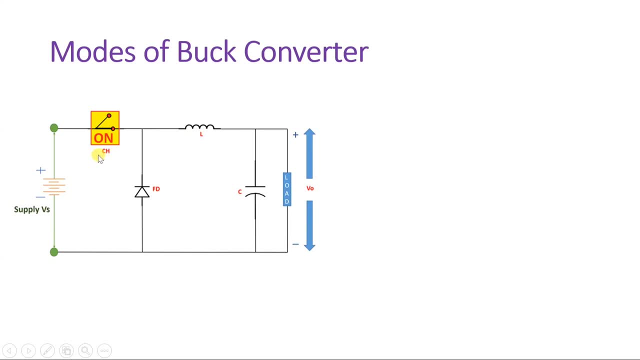 in one mode, switch will be off. So what will happen? as if switch is on. So when you turn on this switch, at that time the supply voltage that will flow current in this loop. So this is the switch that you use for supply current, and when it turns off, current will flow current. 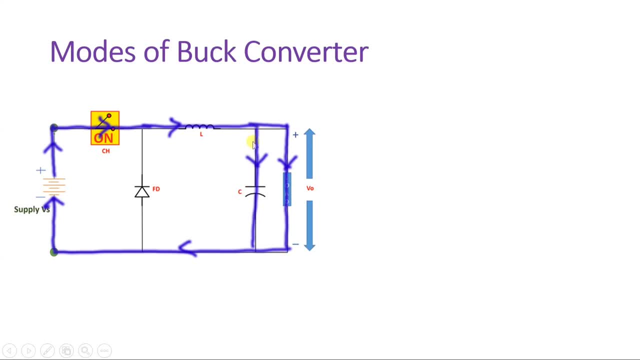 to the AC capacitor. So you can observe, from supply voltage to switch to inductor, current is flowing and current will flow trough the load, As well as partial current will flow in this capacitor. So you can see, as if switch is on, current will flow in this loop When 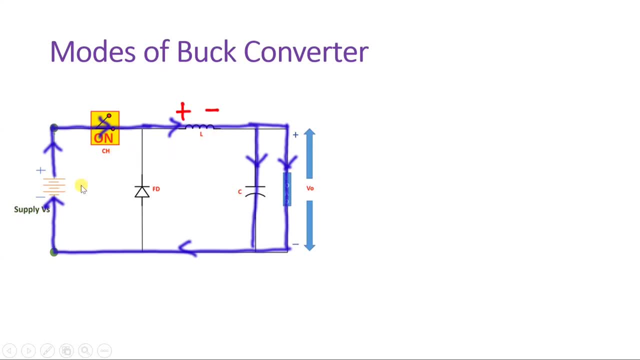 switches off, inductors will get charges and its polarity of Charges will be plus minus, loop through the load as well as partial current will flow through the capacitor, and inductor will get charged by polarity plus minus. so this is what the first mode, which is there with buck converter, 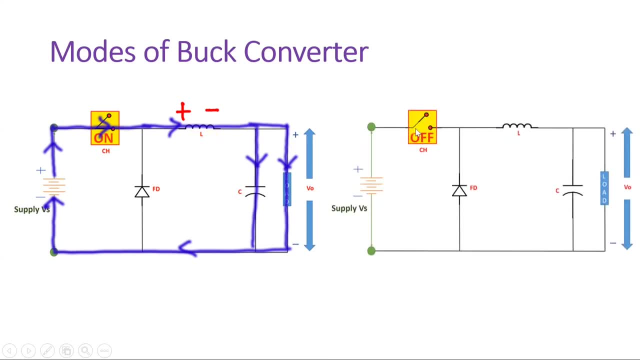 where switch is on. now, what if this switch is off? so when switch is off, at that time the charged energy which is there in inductor, with plus, minus polarity, that inductor will reverse its polarity, so now it will get minus, plus, you can see, and then inductor will release its energy through. 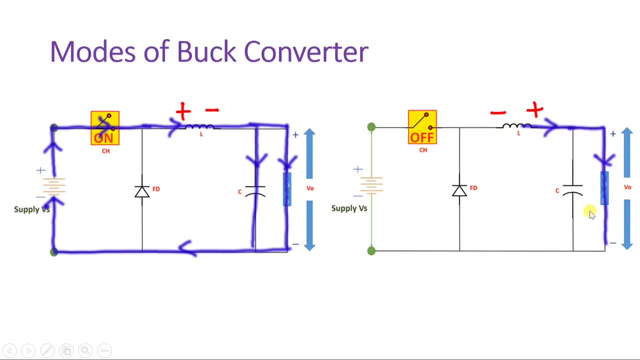 the load. so you can see through the load. current will flow in this loop. so current will flow from inductor to load, to freewheeling diode, and partial current that will even flow through capacitor. so this is how current will flow in this loop you can observe. so there are two modes in one mode. 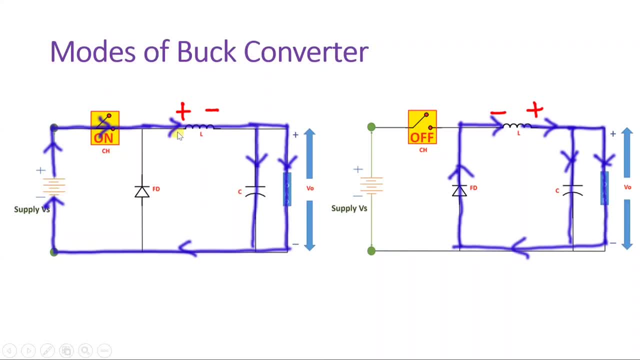 when switch is on and the other mode when switch is off. so this is how current will flow in this mode: when switch is on, inductor will store energy with plus minus polarity, and when switch is off, inductor will release its energy by changing its polarity in this loop, in this case freewheeling. 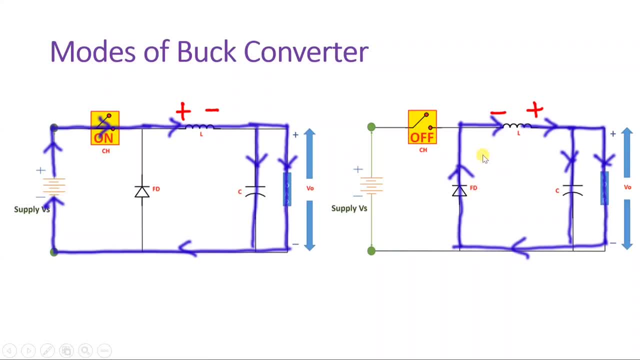 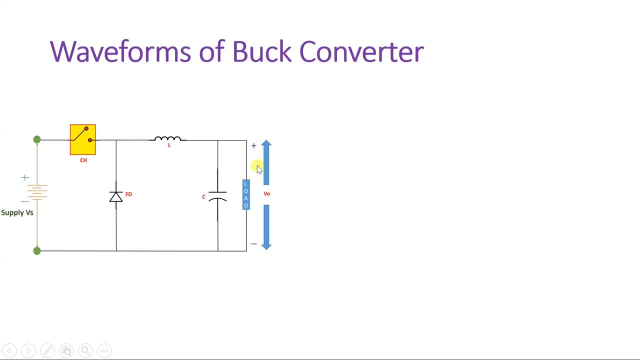 diode will conduct. so this is the modes which is there with buck converter. now let us try to understand waveforms based on these modes. so you can observe, this is the basic circuit and here in waveforms, we are delivered to plot output voltage v0: inductor current, diode current, input current and capacitor current. so here all. 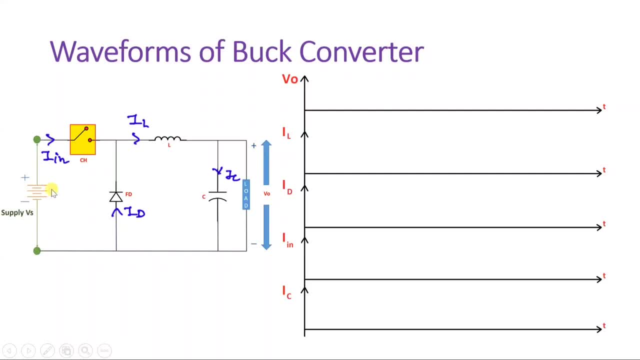 those waveforms that we are delivered to plot based on switches on and switches off. so here i in current that will flow from the supply from here, and this is what il, inductor current will flow current, and this is capacitor current and output current that you can see now, here and when switch. 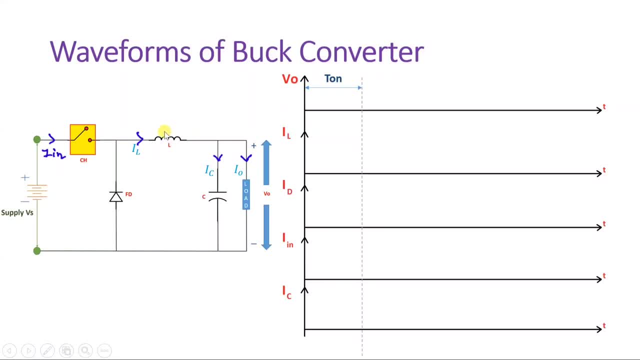 is on, at that time inductor will charge by polarity plus minus, like this. and when switch is off, at that time inductor will release its energy by changing its polarity. so here at output side, first we are delivered to see what will happen when switch is on and what will happen when switch is off. so here 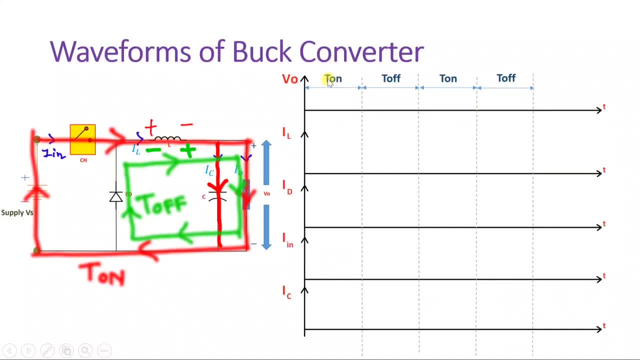 for this time period i have provided turn on operation of the switch and turn off operation of the switch that you can see now, as i have told you, when switch is on, current will flow in this loop and partial current flow will- capacitor that you can see right, and during switch is on, inductor will. 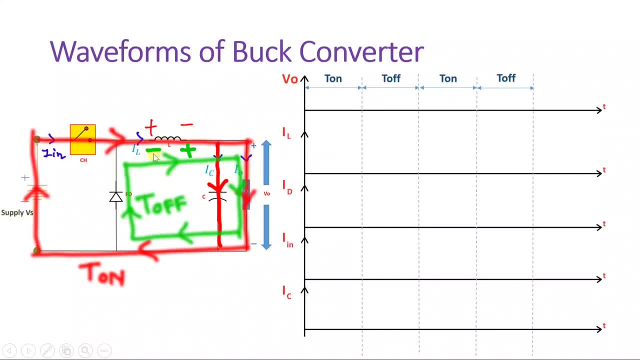 store energy. so current will increase gradually with plus, minus polarity in this direction right, and you can observe at that time output voltage that will appear, which is vs right, or one can say dc voltage, vdc, and when switch is off, at that time freewheeling diode will conduct and inductor will 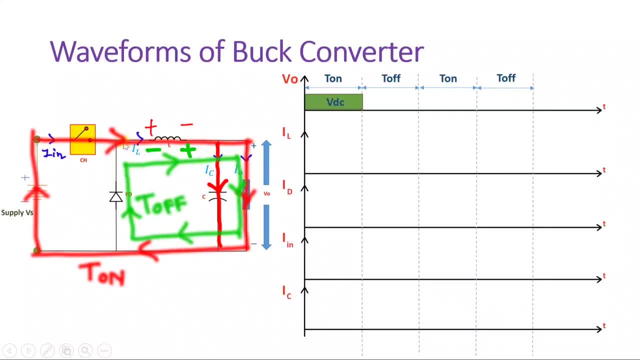 release its energy, so current will flow in this loop. so at that time, as freewheeling diode is conducting output voltage that will be minimum, or one can say zero at load side, so that you can see output voltage that will be vdc during t is on and output voltage is. 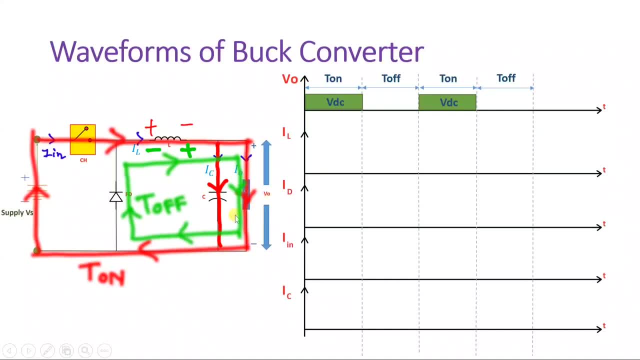 minimum or zero during switch is off. so when switch is on, inductor current will increase from imin to imax, and when switch is off, at that time inductor current will decrease from imax to imin. so this is how waveforms are there across inductor that you can see. so during switch is on, 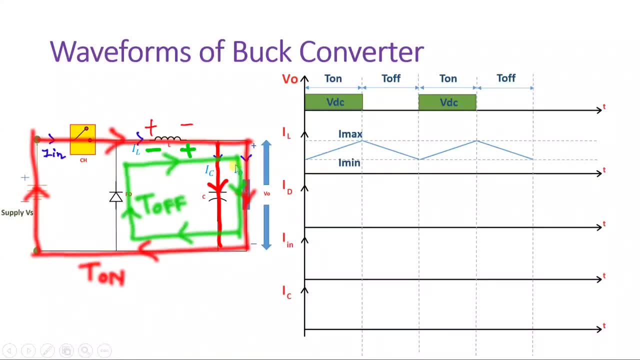 inductor current will increase from minimum to maximum and when switch is off, at that time inductor current will decrease from maximum to minimum. and you can observe when switch is off, at that time this freewheeling diode will conduct. so this diode current that will be appearing during 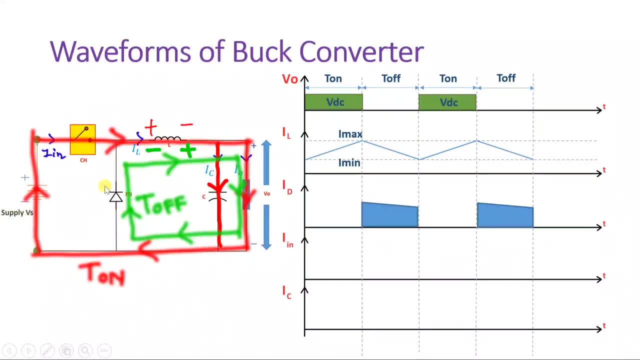 switch is off and when switch is on, at that time freewheeling diode will be in reverse bias, so there will be zero current. so when switch is on, freewheeling diode will not conduct, so current will be zero. and when switch is on, this current of inductor that will appear across diode. 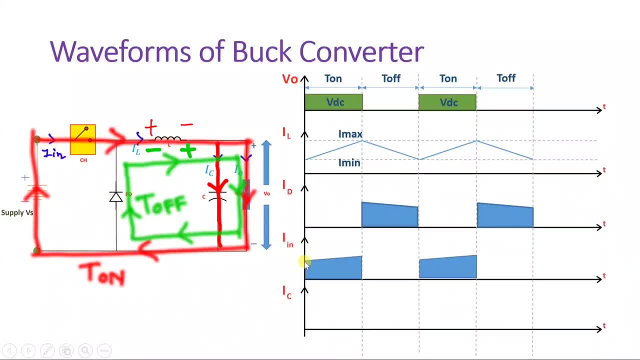 and input current i in current that will appear when switch is on right and when switch is off, at that time this input current that will not flow, so that you can see. so this is what input current which is happening because of vdc during switch is on and this input current is not. 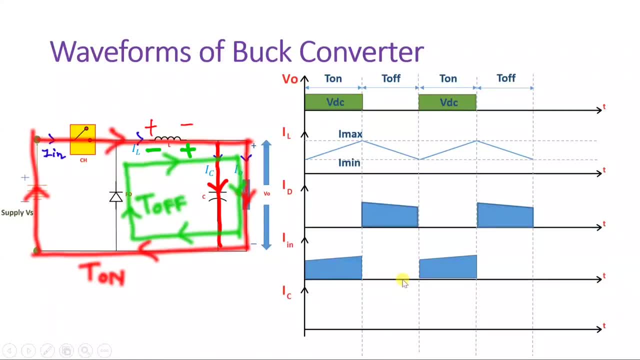 flowing because of switch is off. so it will be zero during t off and capacitor current that will flow like this and it will be having very less value. an average capacitor current that will be zero. i'll show you in calculation how it will be zero. so let us try to understand all those. 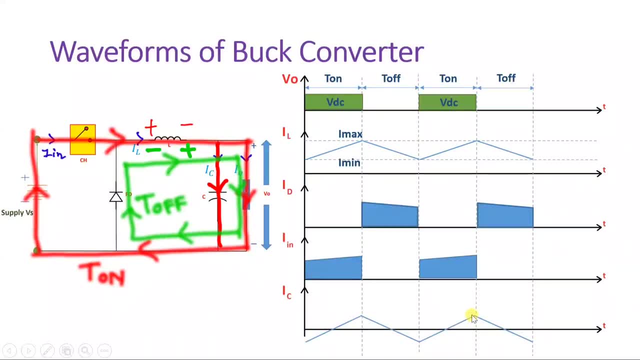 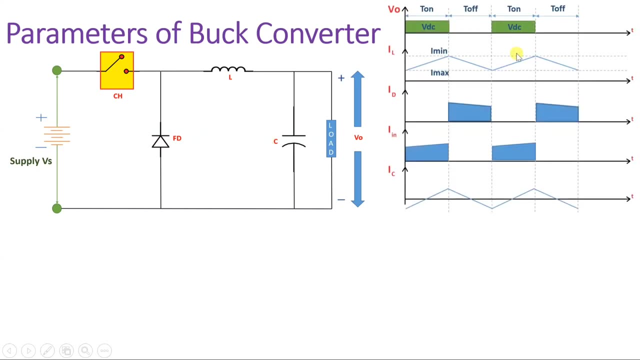 calculation: see capacitor current is happening like this and this average current that you can see it is zero. how it is zero. so let us try to understand that in parameters. so this is the basic circuit that we have already seen and these are the waveforms that i have. 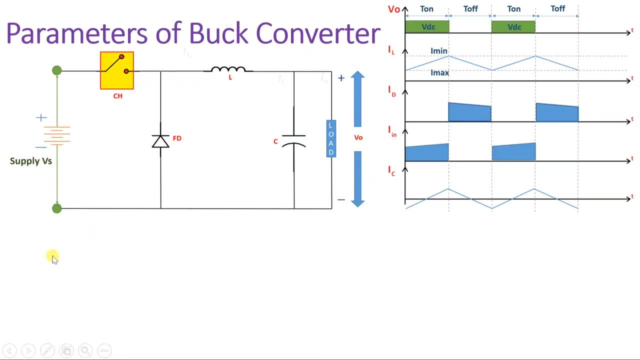 already explained you how that is happening. now, as i have told you what will happen when this switch is on, so as, if this switch is on, you will be observing this current is flowing from supply in this loop, you can see, and this diode will be off. so if you want to calculate, 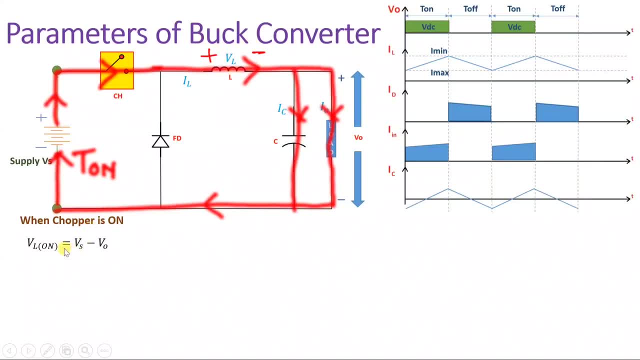 inductor voltage during switch is on, then see this inductor voltage, vl. as per this loop you can say this vl will be vs minus v0. and if you calculate ic current, then if you apply kirchhoff node loop at this node then this is il current, then ic on current that will be il minus iz. 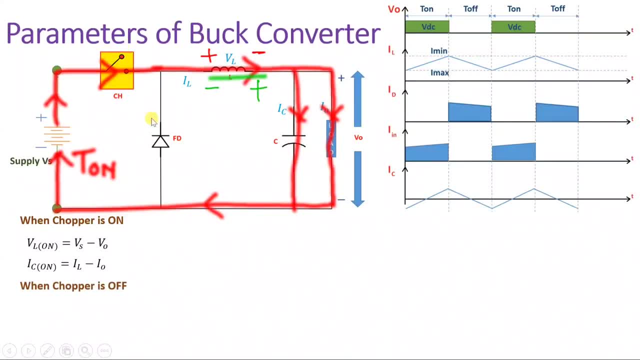 and when this switch is off, at that time this inductor will release its energy and current will flow in this loop. so you'll be observing this vl voltage plus v0 voltage. that will be zero. so we can say vl off voltage, that will be equals to minus v0. and regarding ic off current, we can say it is il. 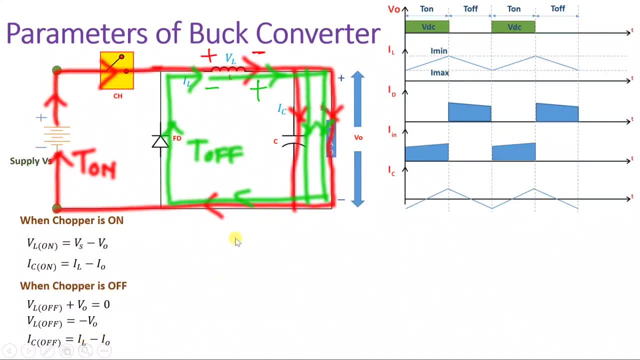 minus i0. now, based on this, we will apply volt second balance. so see if we apply volt second balance across inductor voltage, then we can say vl on into t on plus vl off into t off, that is equals to zero and vl on that we have calculated. it is vs minus v0 and vl off. that we have calculated. it is minus v0, so that is placed into the loop and that way you are able to say the current of this Erfolg or the voltage matrix is not telefoting. we are able to calculate the voltage across the delt Crux upon a current if any of the two calculation. Wahl 미. 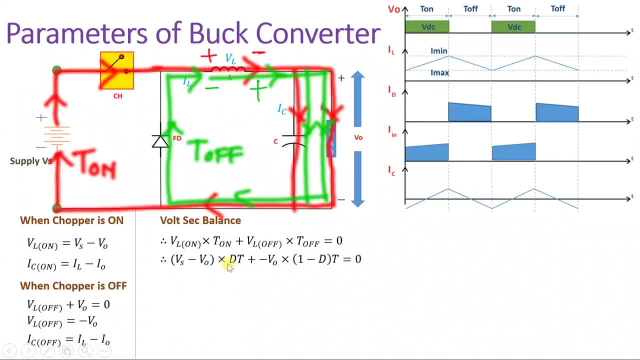 it over here- and t on, that is duty cycle into t. now that we already know like, see, duty cycle is t on divided by t, so t on is equals to d into t- that you can see it over here- and t off, that is 1 minus duty cycle into t. and if you solve this, then you will be finding it is v. 0 is equals to 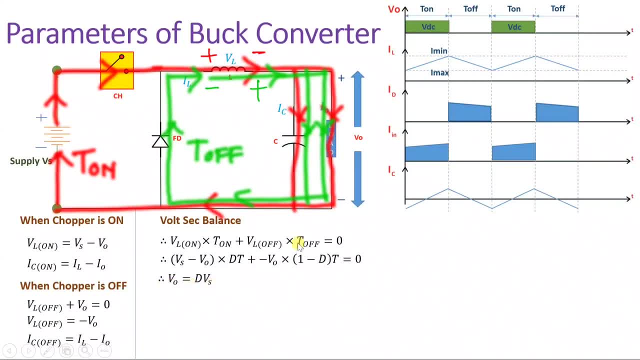 duty cycle into vs. so our average output voltage in this buck converter that is duty cycle into vs. now you see duty cycle range that is there from 0 to 1. it cannot be greater than 1. so duty cycle is 0 to 1. so output, average output voltage that is always less than supply voltage vs. so here 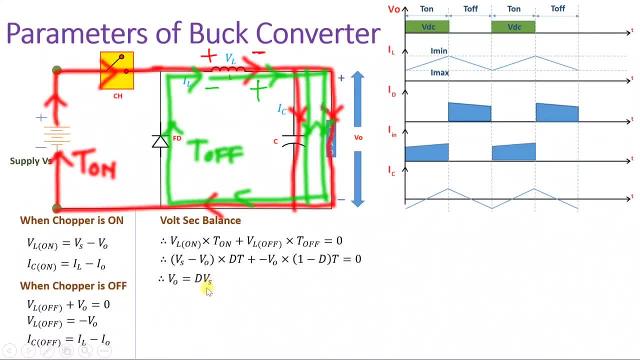 average output voltage is always less than supply voltage vs. we can say this is a buck converter. so here duty cycle is always less than 1. it is ranging in between 0 to 1. so this type of chopper is referred as step down chopper and even this converter is even referred as buck converter. 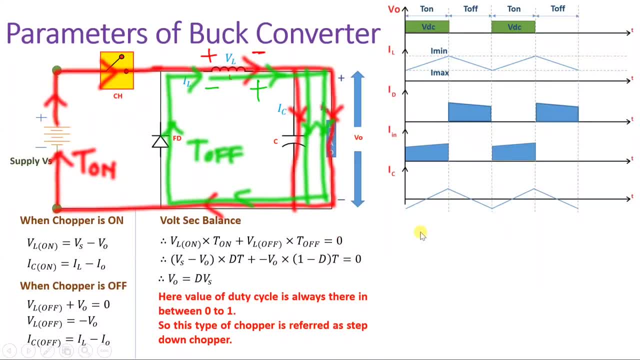 Now let us apply current second balance. so if we apply ampere second balance, then that ampere second balance now that we will apply it for capacitor current. so capacitor current during on into t on plus, capacitor current during off into t off, that is equals to 0. 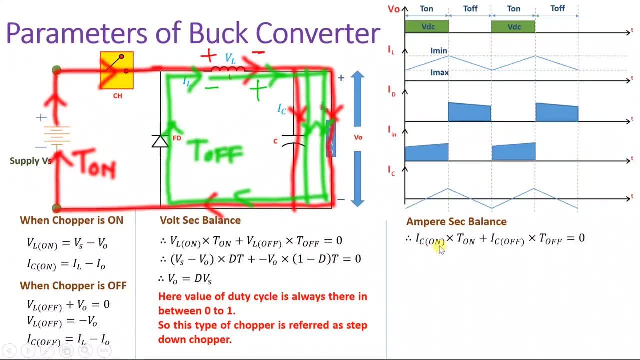 as per ampere. second balance. So IC on into t on plus IC off into t. off, that is equals to 0 and IC on, that is IL minus I0 and IC off, that is even IL minus I0.. So if we apply this and if we resolve this equation, then you will be getting IL is equals. 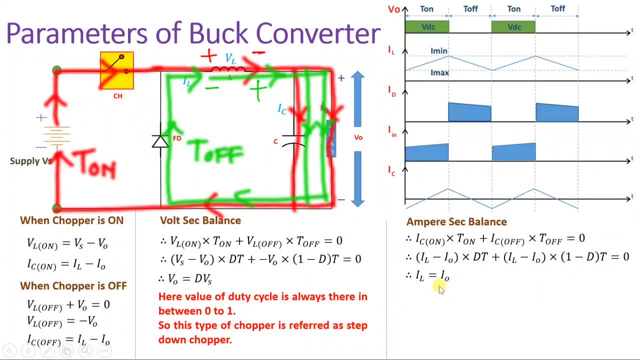 to I0.. So as IL is equals to I0, you will be observing average DC current of capacitor that is zero. Why the reason is: IC is equals to, IC is equals to IL minus I0. and if IL is equals to I0, what it means? average IC current through capacitor that is zero. 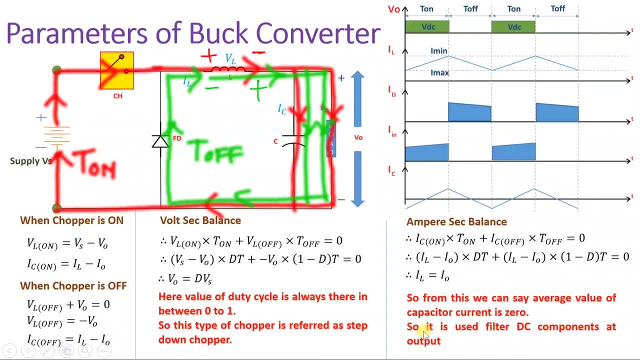 So from this we can say average value of capacitor current is zero. So we can say it is being used to filter DC component at output side, but average current through capacitor will be zero. So in so many books you will be finding this capacitor current is not drawn but that capacitor